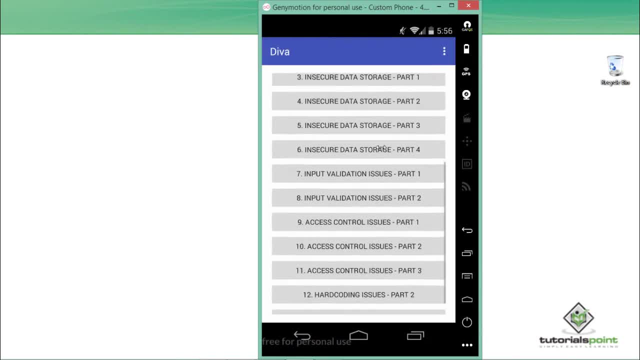 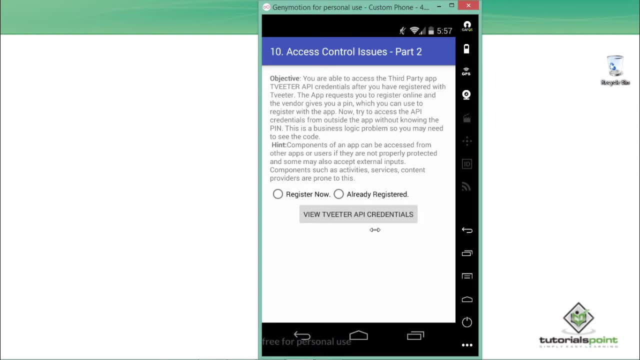 Deva, so let me open it up. and you can see here one issue called as access control issue, part 2, so let me open it up. So this issue is same like the previous one, whereas here, in this issue, what we have to do in order to view API credentials, we have to register at piatucom. so you can see here. 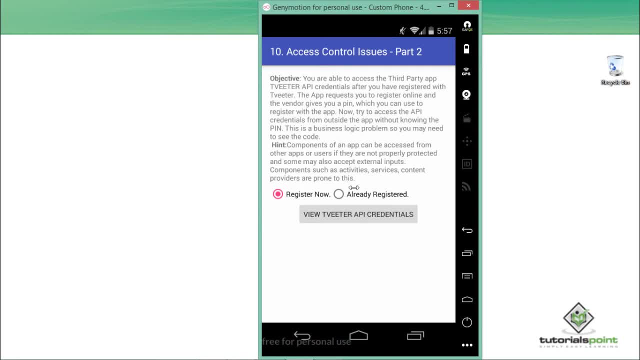 there are two options. the first one is register now and the second one is already registered. so if we click over here, register now, and if we click over here, view Twitter API credential so you can see here, then it asks us for registering at piatucom. 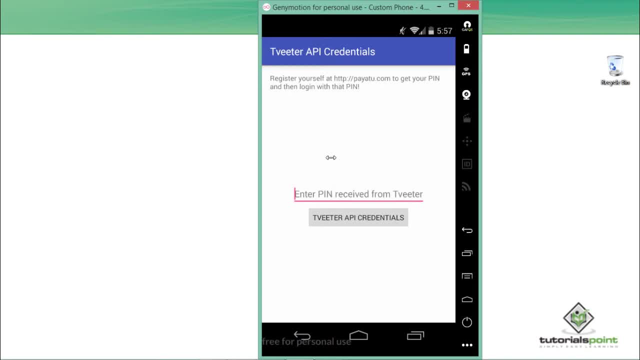 In order to get a pin. so once we get a pin we have to enter over here and then we can able to login, whereas in the second scenario. in the second scenario there is an option of already registered. so if I click over here, already registered, and if I click over here. 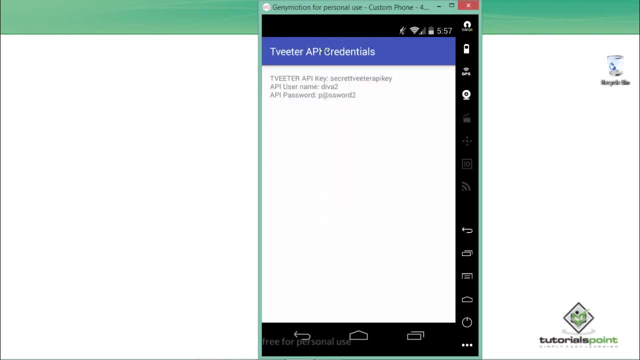 now view Twitter API credential. you can see we are able to access the Twitter API credentials. so what actually happening is, if we click over here, already registered, then our application assumes that we already registered. We already have a pin. it's just a fictional. so what we have to do here is we have to directly. 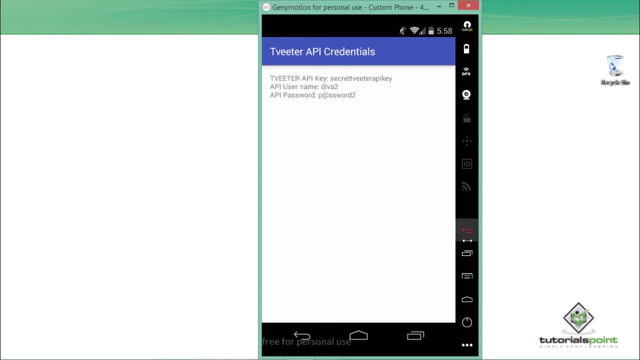 invoke this activity or this Twitter API credential outside the app. so you can see here: it's same that you are able to access the third party Twitter API credentials after you have registered the Twitter. the app request you to register online and the vendors give you a pin. then 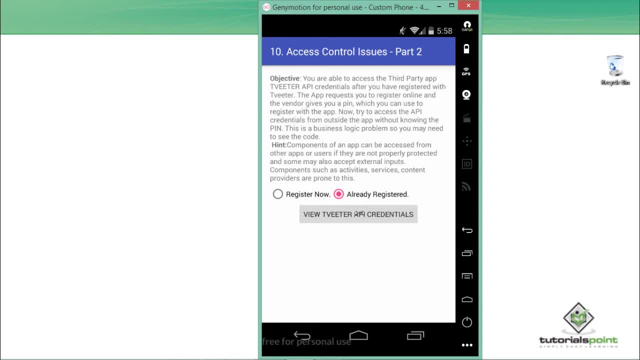 what we have to do? we have to try to access that Twitter API credential without knowing the pin. Now what? What we have to do here is: I am going to invoke the same activity of this Twitter API credential by using activity manager. then we will see that, whether we are able to invoke it or not, 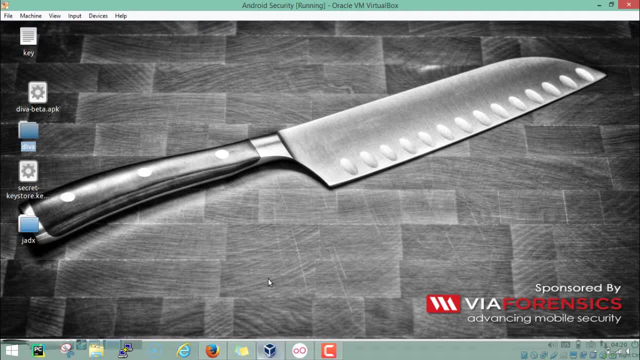 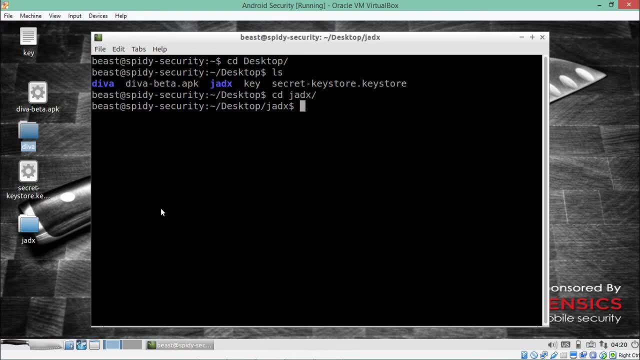 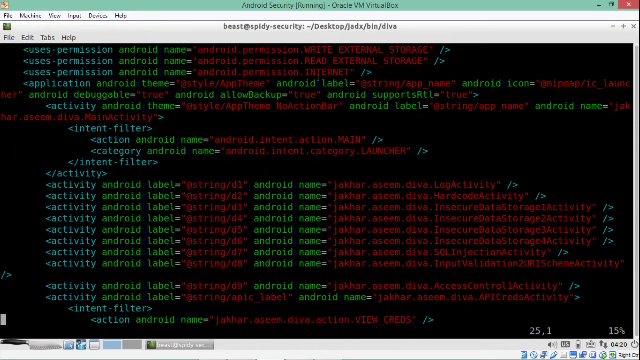 so let me close this up so you can see here that our Centuco VM operating system is up and running. and now let's go here on my desktop, let's go inside. let's go inside ZX bin diva and now let's analyze this. Here is the Android manifestxml file, so you can see here a list of activities and the 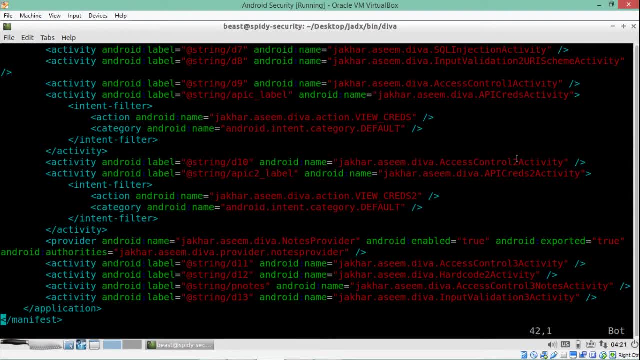 first scroll down. you will find one activity named as access control to activity, and right below it there is one more activity called as API credential to activity, and right below it here is our intent filter. So the name of intent filter is jakhaasimdiva. 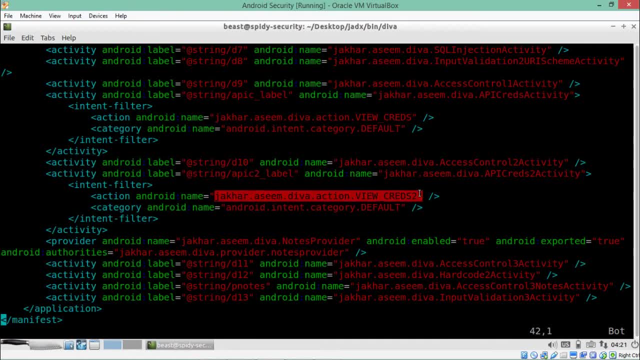 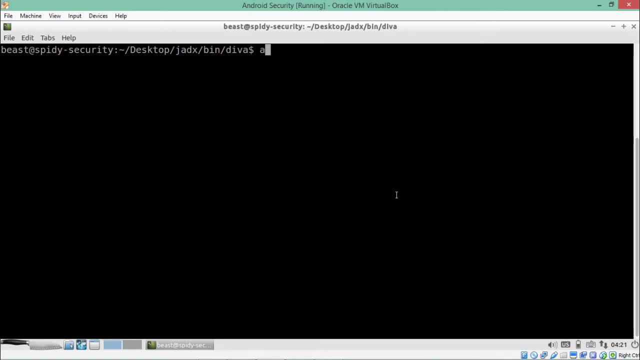 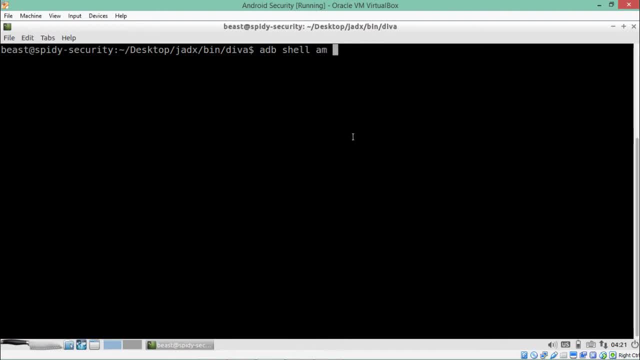 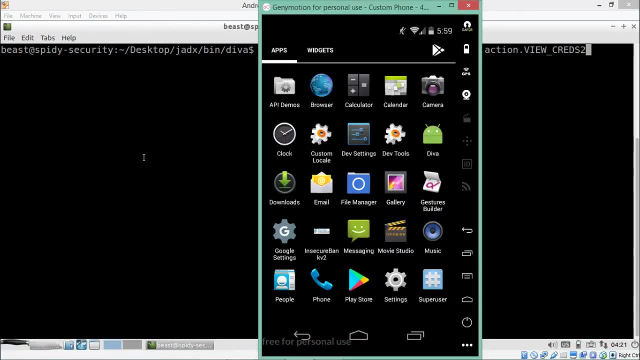 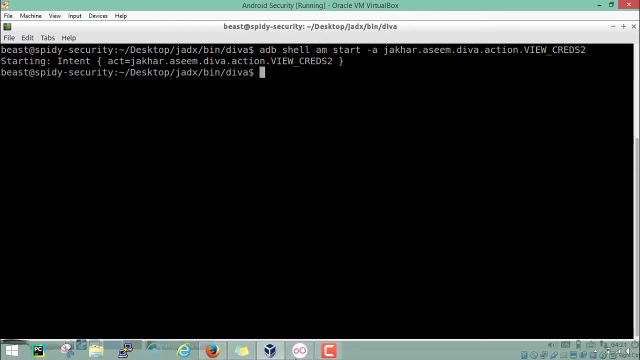 filter by writing over here: adb shell. then activity manager start hyphen A and let me paste intent filter over here and you can see our Genymotion. So if I click on enter you will see that it has started a particular activity and if I open my Genymotion, 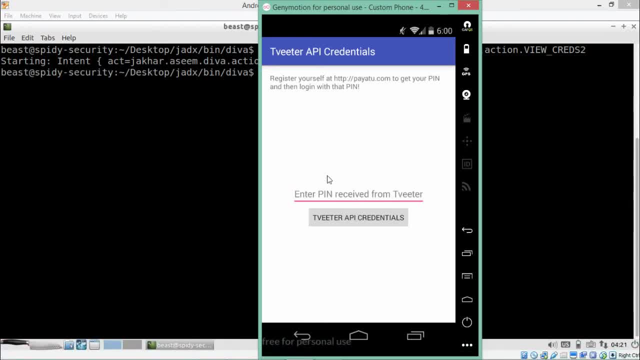 You can see that it's again asking for entering a pin, which means this application or this issue- that is, access control, issue part 2- is actually protected, which means we are not be able to view the Twitter API credential without entering a pin. means it's a compulsory. 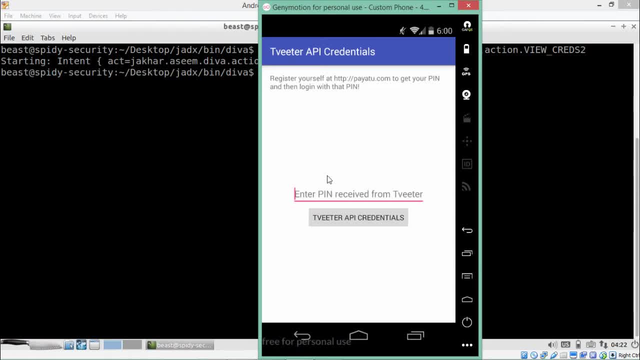 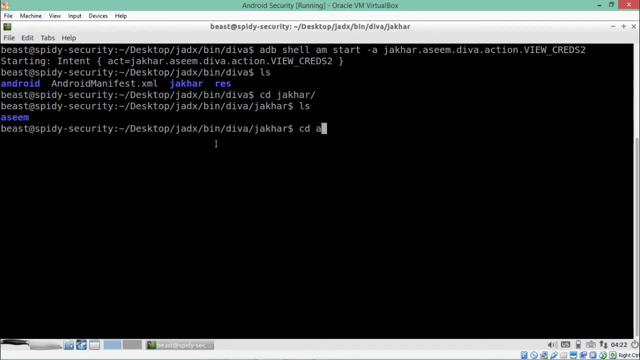 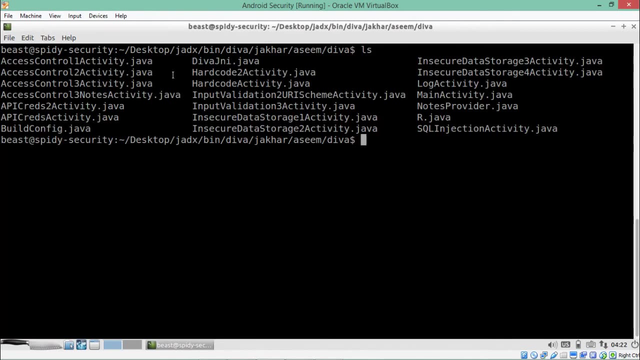 that we have to enter a pin Now in order to bypass this issue. let's analyze its source code. So let me go inside this package. that is jakhaasimdiva. so we have decompiled this application in the previous video. that's why I am able to view the source code, so you can see here one. 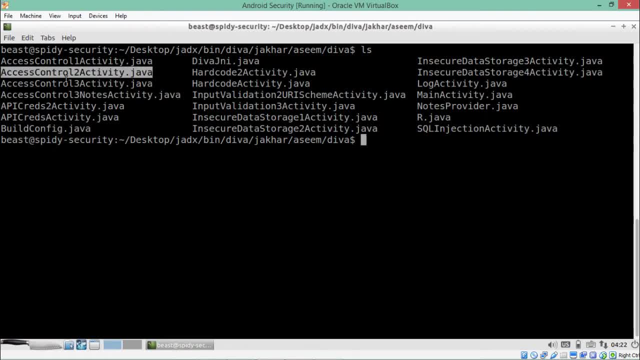 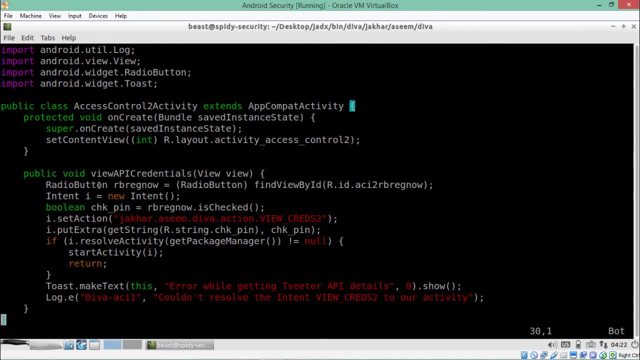 activity called as access control 2 activity. so now let me view its source code. okay, so if I scroll down, you will see one function called as view API credentials, and here the thing to be noticed is that there is one variable or a string called as chkpin, which means check pin, and it's a boolean one. that is true or false, as. 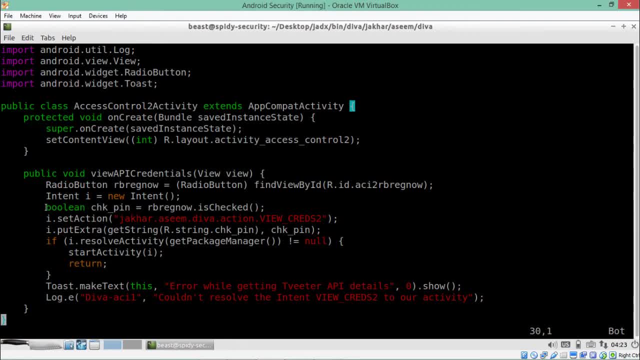 we all know that boolean operator might be a true, might be a false. so here you can see that there is one variable or a string called as check pin and that's a boolean. so what actually happening is you can see if else statement over here, that is, if statement. so 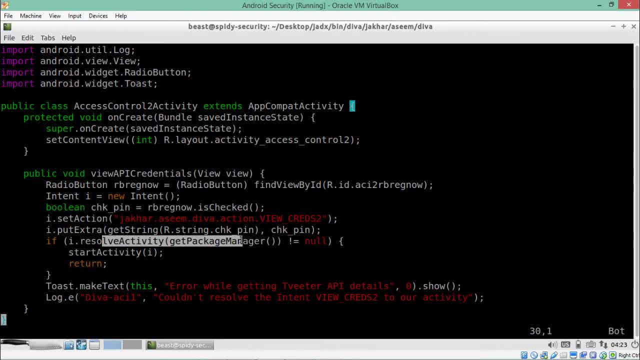 if the string that we entered or the pin which we enter, so if that is not equals to null, then what happen is it will display the same activity, whereas if this pin is not equal to null or it's a null, then what happen is it show us the twitter API credentials. now. 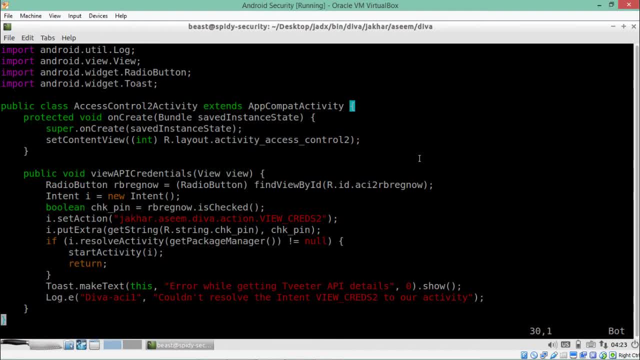 what we have to do is, in order to invoke that particular activity, we have to pass one another parameter called as chkpin. The thing to be noticed is that this chkpin is not actual string, so if you are a android developer, you might know about stringsxml file, which contains a reference of strings. 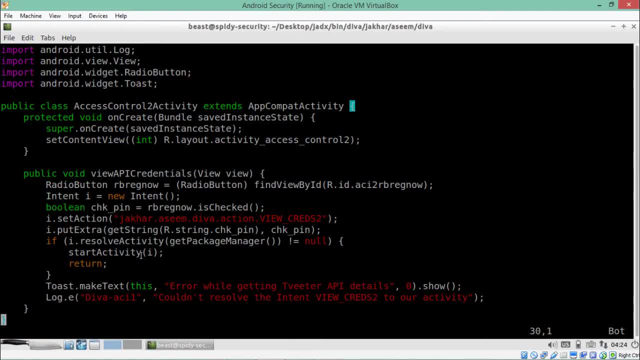 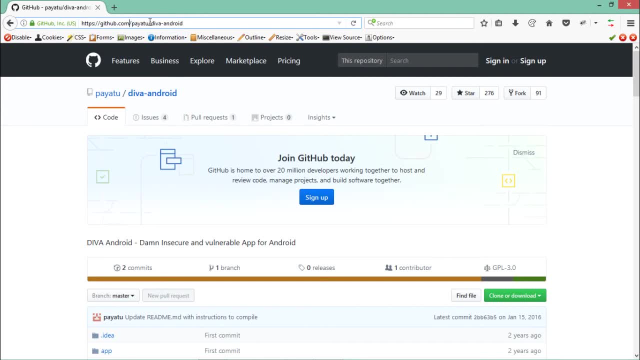 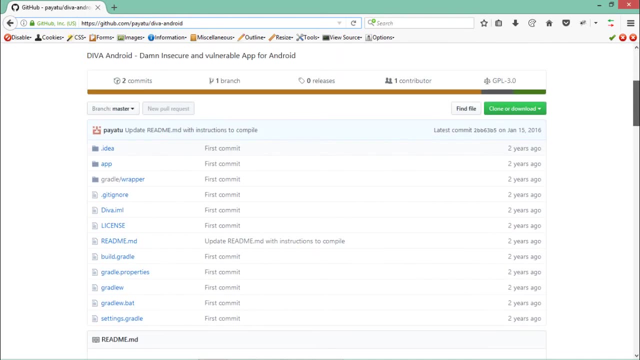 so actual value of this variable is something different. so in order to view it, let me go here to its github link, that is githubcom: slash, py2, diva and diva slash android. so from here you can download the source code of this application. that is diva. so in order to view, 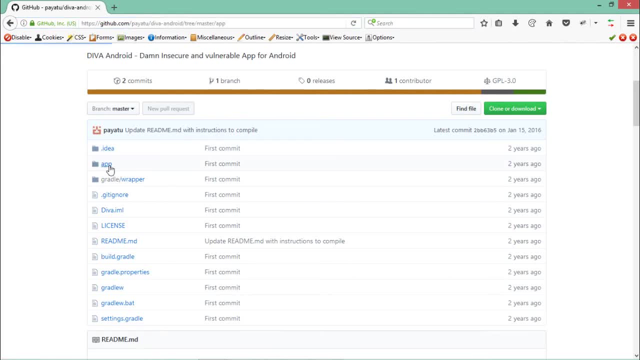 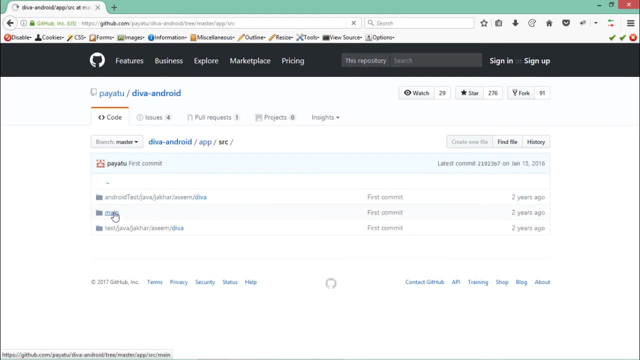 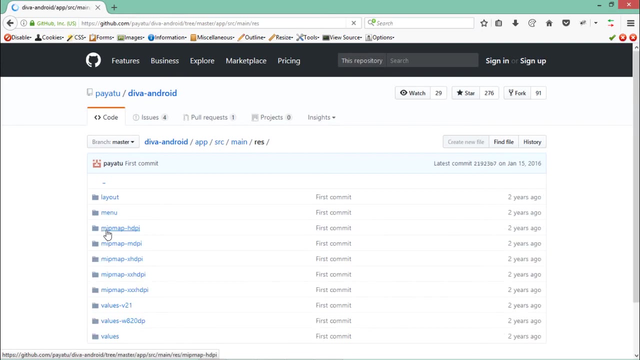 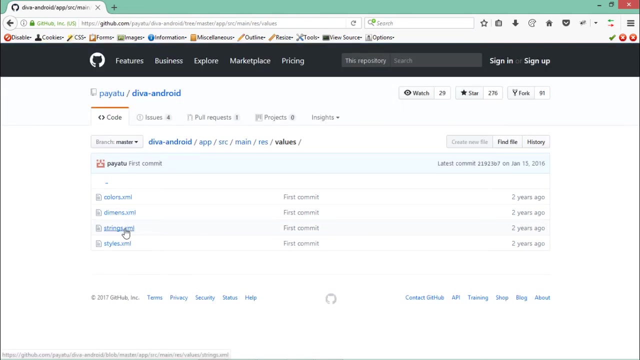 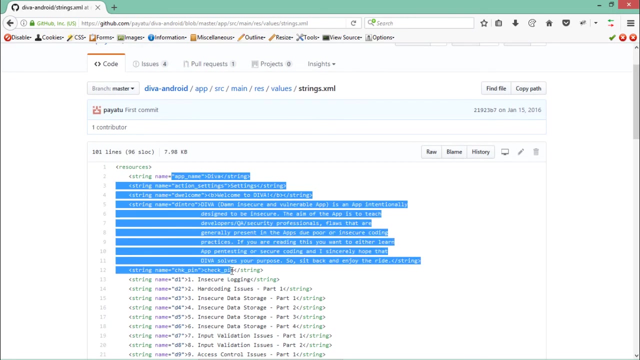 stringsxml file. let's go inside over here, app source main, and here is one directory called as res- that is resource, so let me open it up- and values- and here you will find one xml file called as stringsxml, So you can see here all the strings with its values. so you can see here that wherever inside. 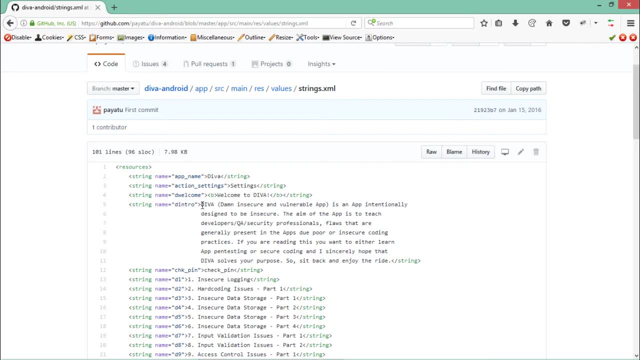 the application this is written dintro, which means if in application this keyword is written, then it reference or it points to this entire text. now let's try to find chkpin. so you can see here our chkpin string. but the exact value is checkpin, so that is ch, e, c, k pin. so what? 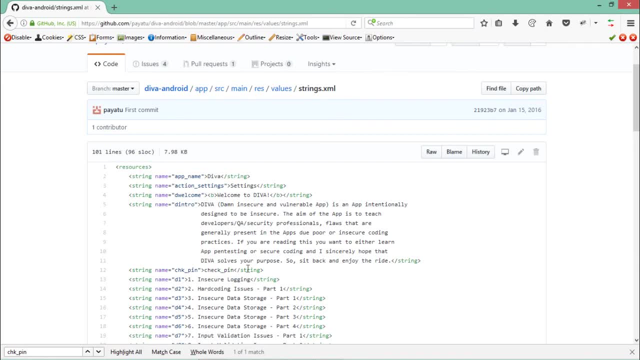 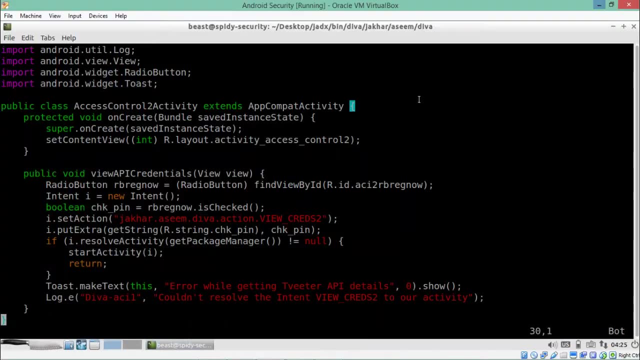 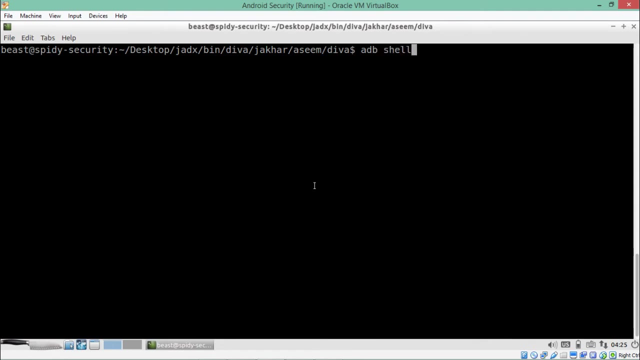 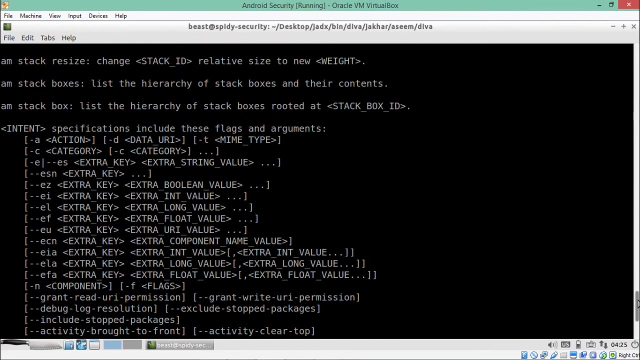 we have to do here is Now, in order to invoke that particular làthivity, we have to pass this ch, e, c, k checkpin parameter. so first of all, let's go inside adb shell and let's see how we can pass parameter in activitymanager. so I'm just writing here am. so you will see here that, in order to start, 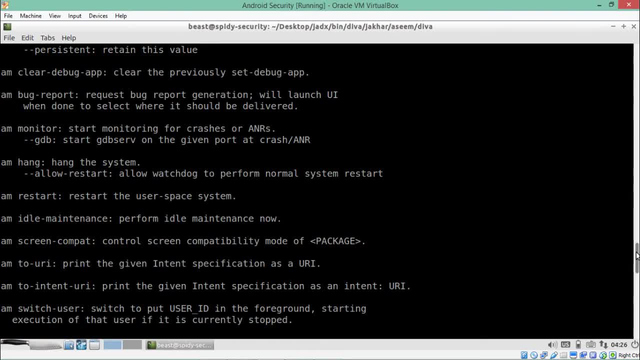 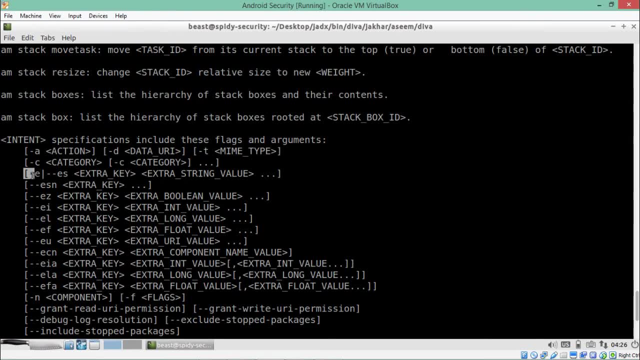 any activity have to write am start hyphen a. but now let's see how we can add parameter. so if I scroll down you can see here the first option is hyphen e. so by adding a hyphen e we can pass a parameter. but that will be a string. so if we write here hyphen e, z, then we can write. 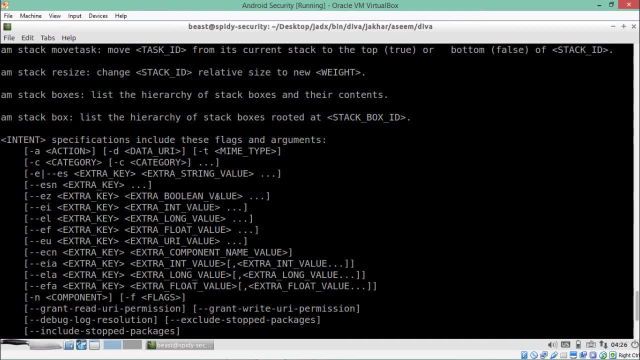 any parameter and we can give its boolean value. similarly, if you want to pass any particular parameter that takes integer value, then you have to use hyphen ei, whereas hyphen el used for extra long value, but for the time being we are interested in this parameter, that is. 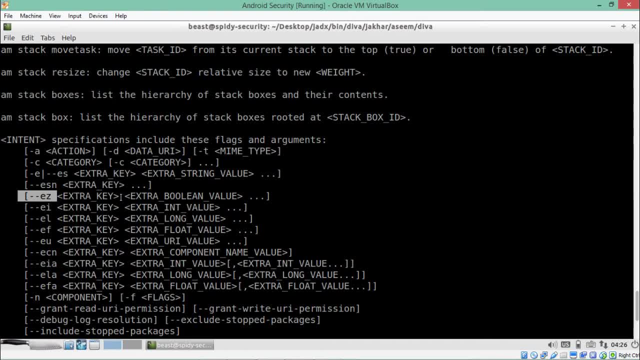 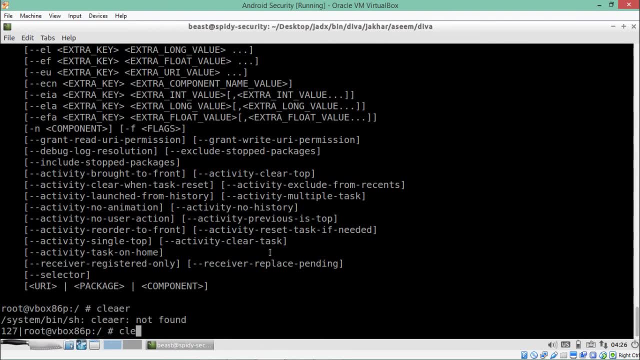 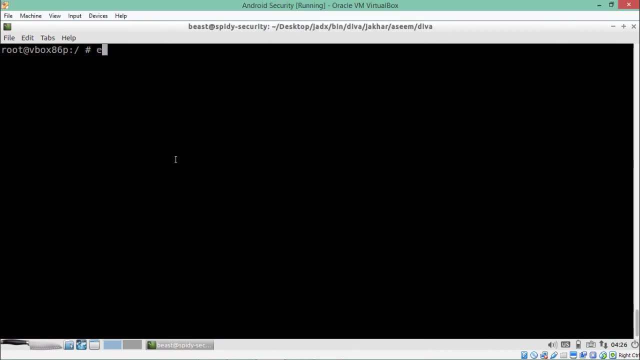 hyphen, hyphen e z, in which the hyphen e z actually supports boolean value. so now what I am going to do here is: so let me first of all close this div application, so let's just write here and let me go back close this genymotion shell. now you can see that right now we are inside the centochrome embedding. 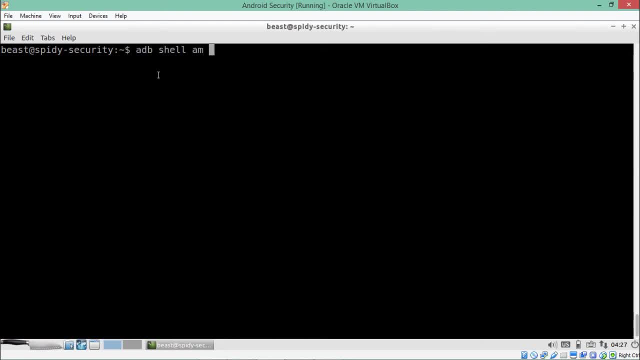